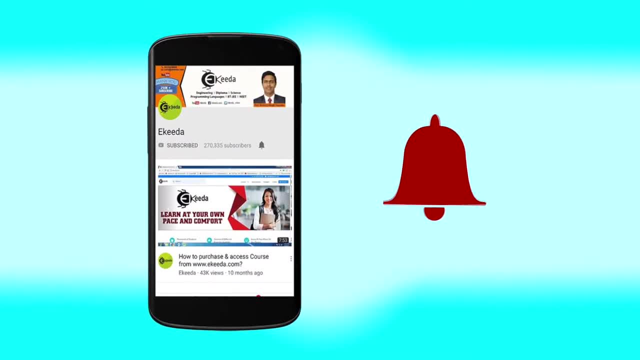 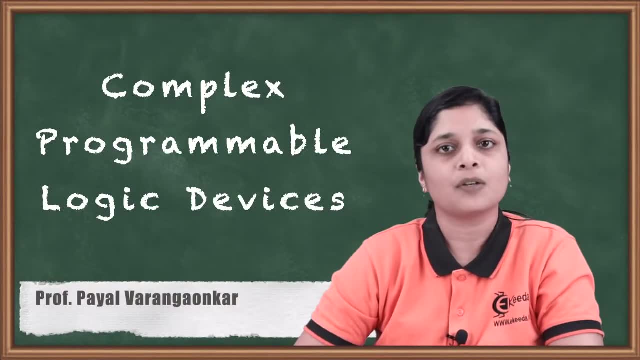 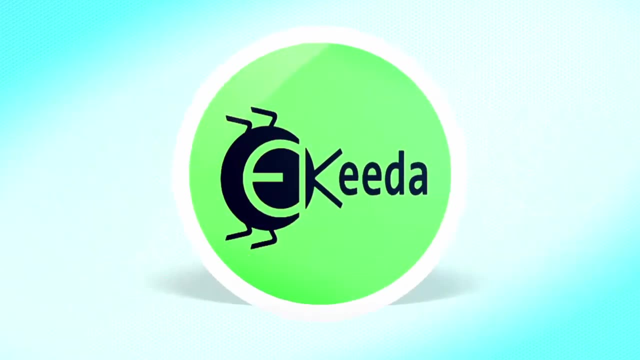 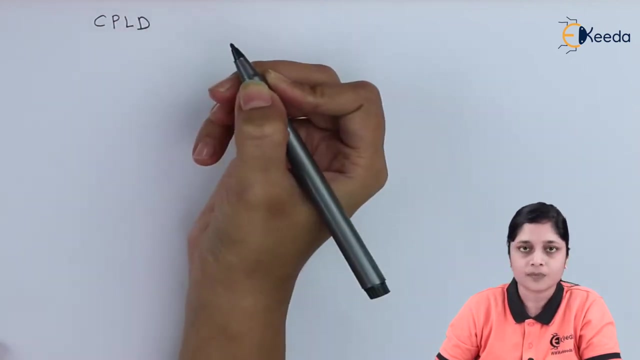 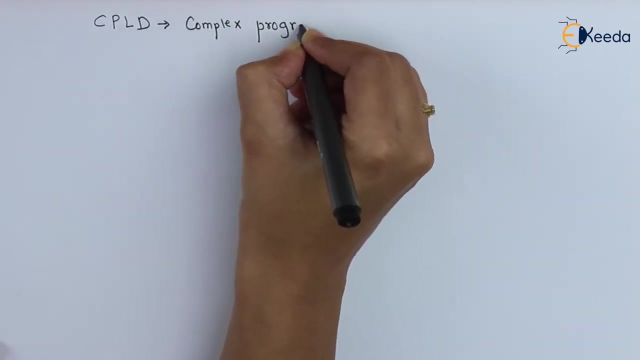 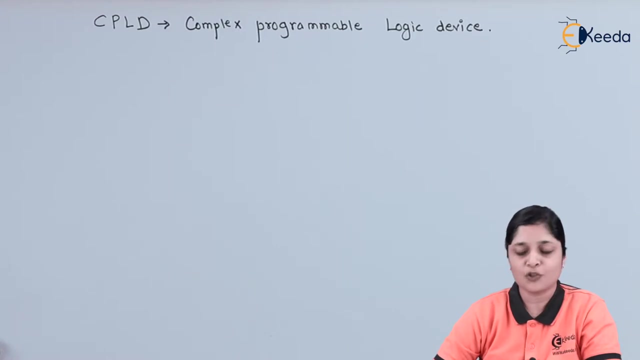 Hello friends, now we are going to discuss the CPLDs, ie Complex Programmable Logic Devices. So we will discuss here the CPLDs. First of all, we will write its long form: CPLD stands for Complex Programmable Logic Devices. 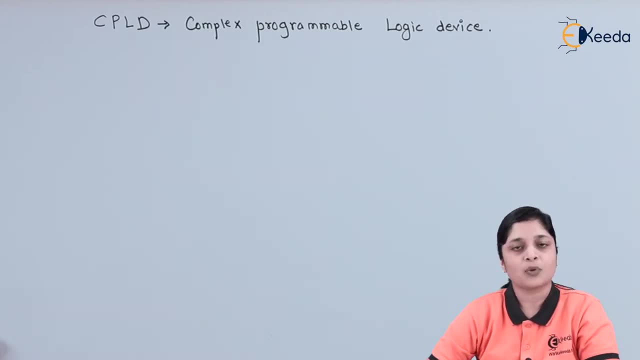 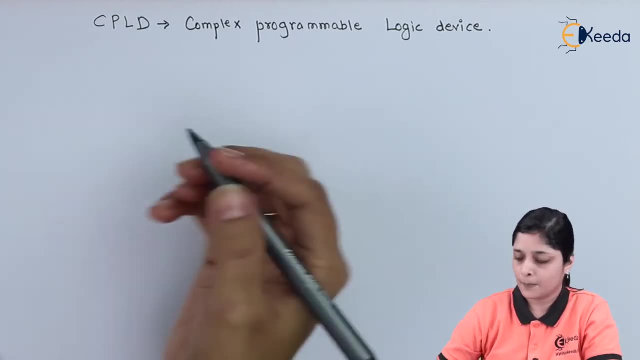 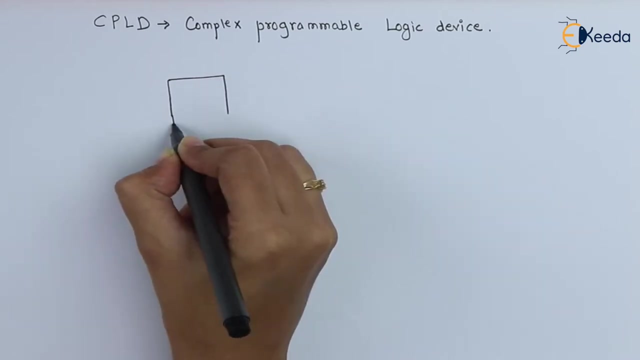 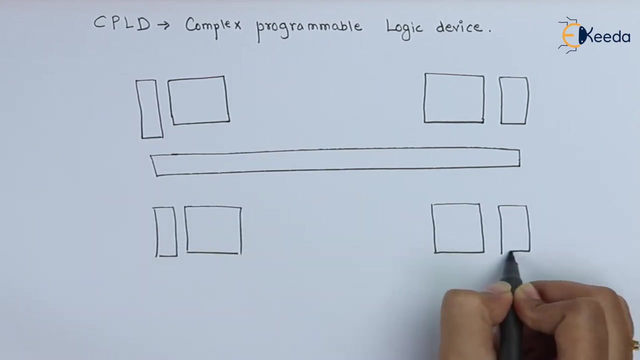 It is a type of PLDs, ie Programmable Logic Devices. Now we will discuss its logic diagram first of all. So if you consider the logic diagram, it consists of many number of PAL-like boxes, So we will label these boxes. 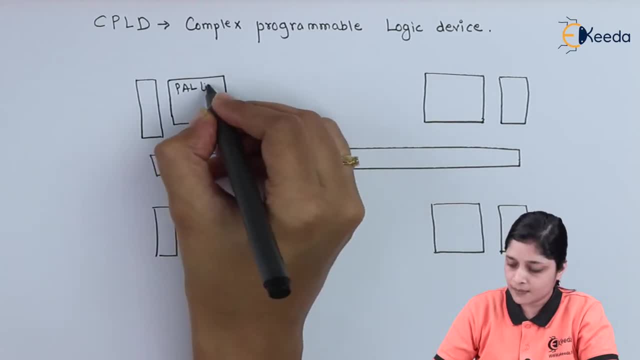 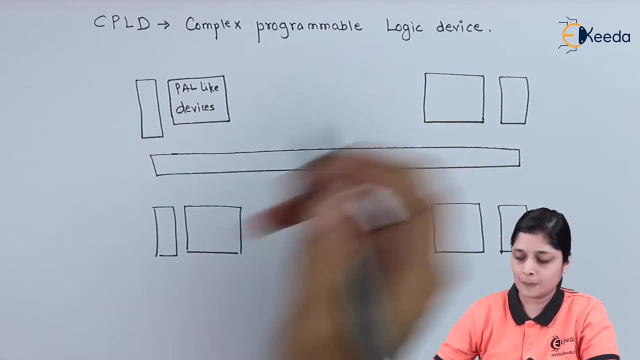 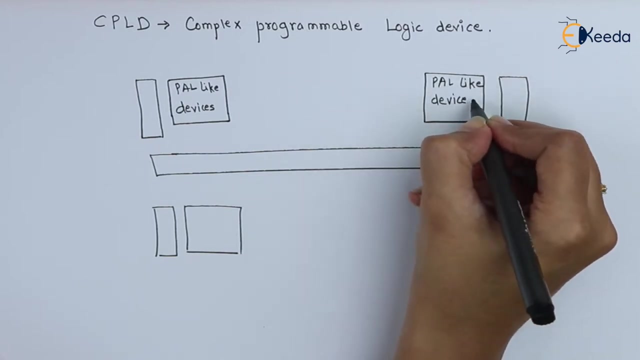 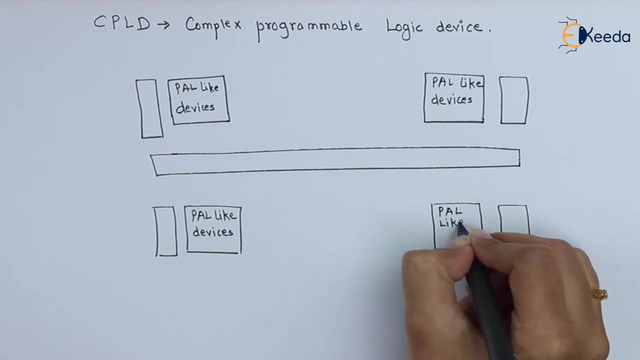 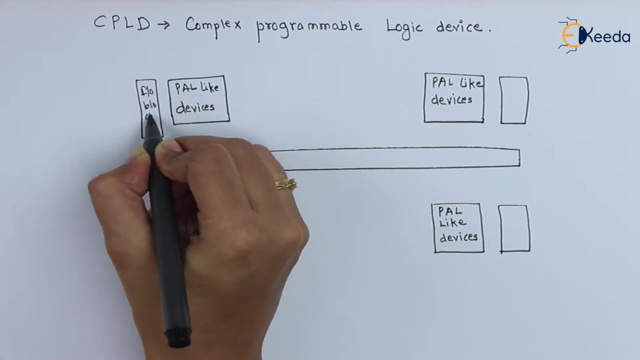 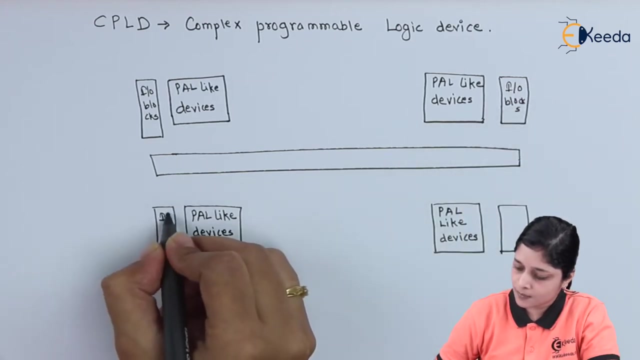 This is your PAL-like devices. It can be PAL or PLA. It can be PAL or PLA. So, all these are your PAL-like devices. These are your I-O blocks. All these blocks are I-O blocks. All these blocks are I-O blocks. 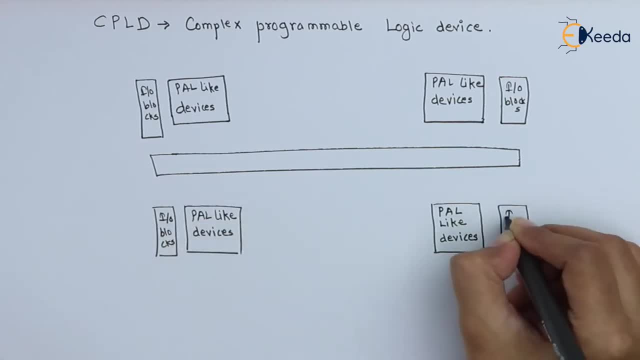 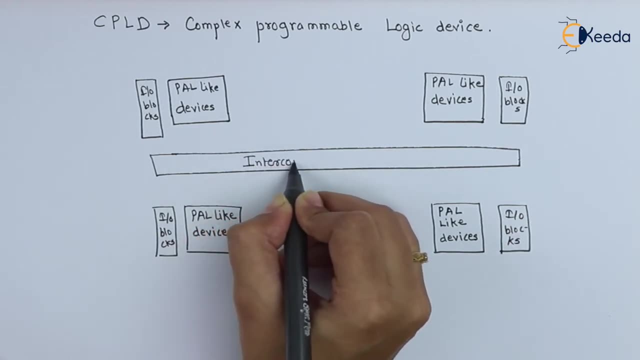 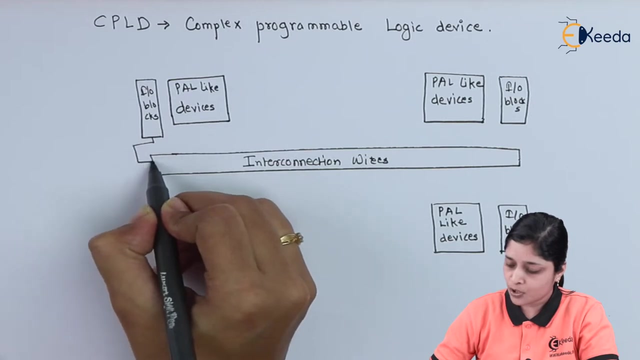 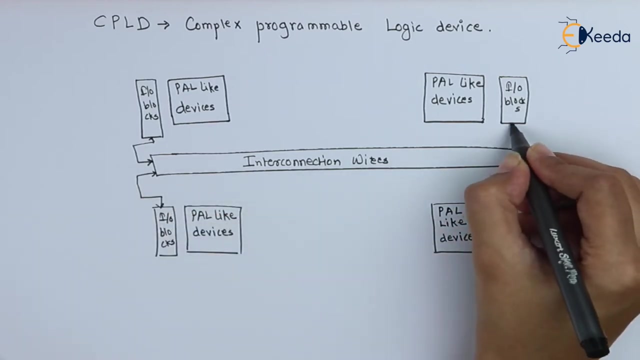 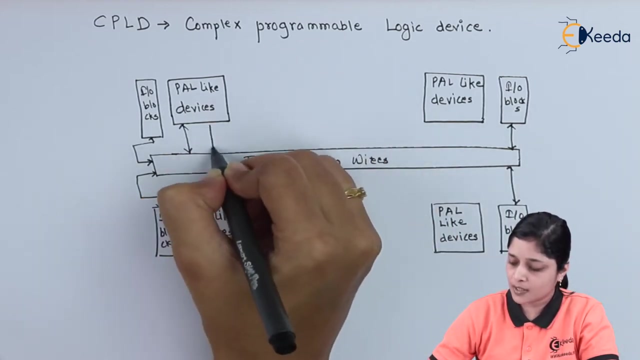 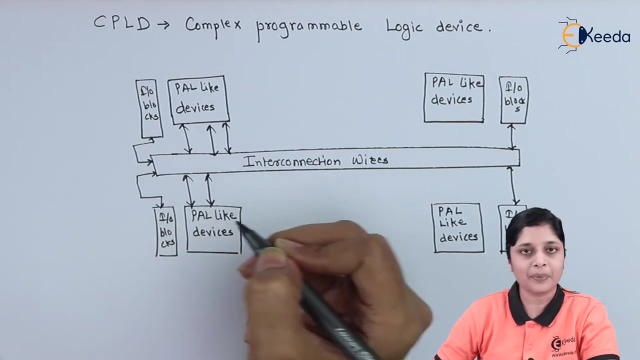 That is input, output, And this is the interconnection wires. Now all these boxes are interconnected, are interconnected Like this, Like this, And these devices are also connected to the interconnection wires. These devices consist of PAL or PLA.